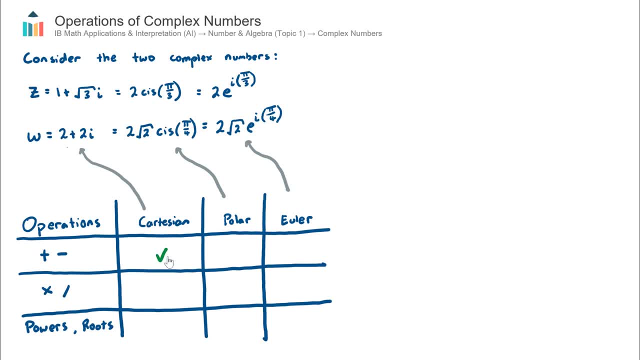 green tick here, next to the addition for Cartesian form As opposed to polar and Euler form. in order to add or subtract complex numbers in polar or Euler form, we need to convert it back to Cartesian form anyway in order to perform that operation by hand. So I'm going 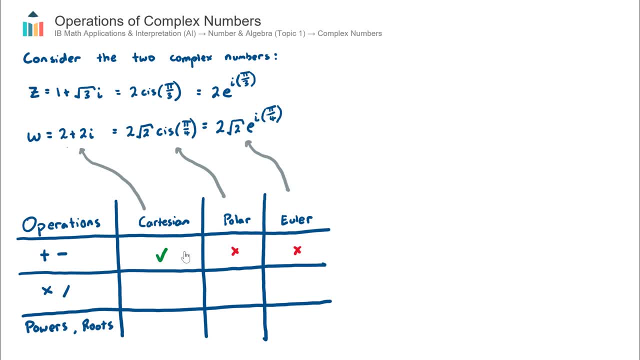 to put two crosses here. So let's demonstrate now how to add these two complex numbers together, Z and W, in Cartesian form. So Z plus W is equal to, and the way that we do it is adding the two, the real components, together. So the real component of complex number Z is 1 and the 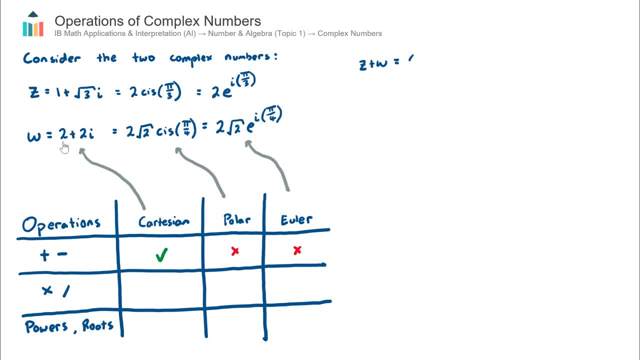 real component of complex number W is 2.. So this will be 1 plus 2 plus. and then we add the imaginary components together, So root 3 plus 2.. So this will be root 3 plus 2. And because these are the imaginary components, it will be root 3 plus 2i. And if we add the 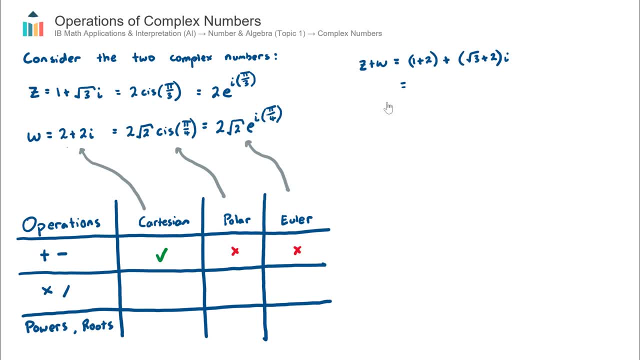 terms that we can add together. so we can add the 1 plus 2 together, this will be 3 plus. but we can't add root 3 plus 2 together, so we're just going to leave this as 2 plus root 3i. 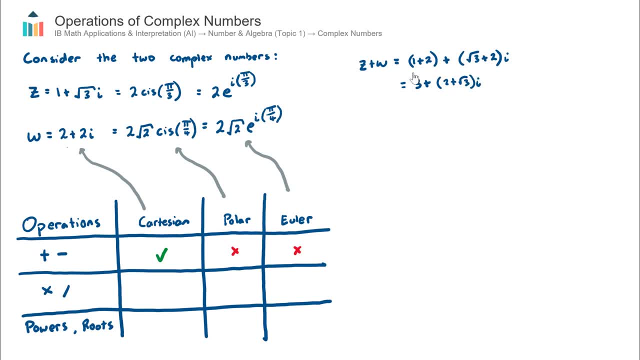 So there we have it. We have added the two complex numbers together. Now we're going to add the two complex numbers together. So we're going to add the two complex numbers together. Fairly easy to do. The subtraction is the same process. I won't go through that. 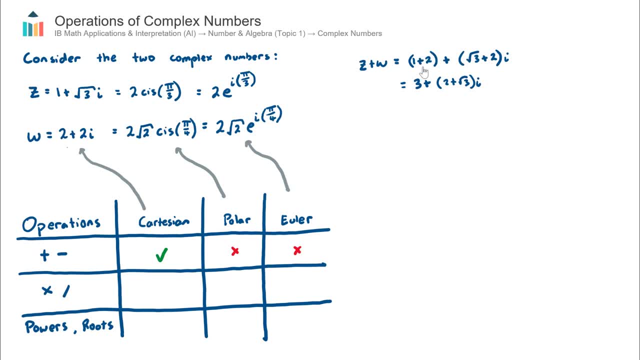 but for subtraction. we just subtract the real components from each other and also the imaginary components from each other. So that's all that. it is to it there for addition and subtraction. Let's now move on to multiplication and division. Now, multiplication and division can actually 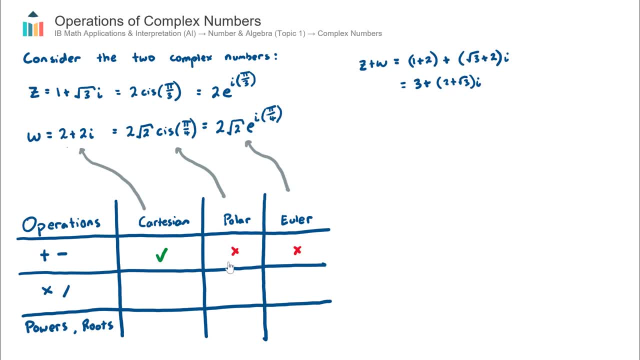 be done in either of the three forms. However, I will preface it that although you can multiply two numbers together or divide in Cartesian form, it starts to get quite complicated if you have, say, more than two complex numbers Or if the complex 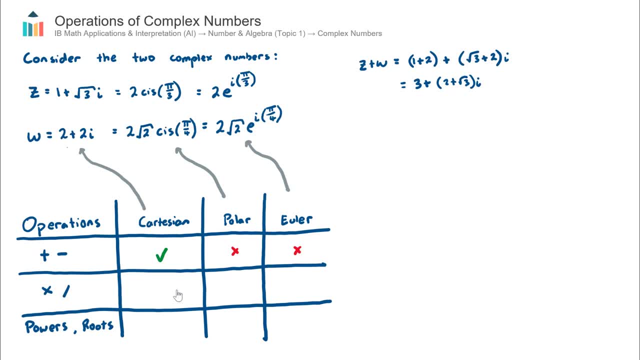 numbers are quite difficult. they're quite sort of complicated or tricky. Cartesian form becomes a little bit harder to do, Whereas polar and Euler form still will be quite easy to do. So let's demonstrate all three processes and then, I think, through it you'll start to. 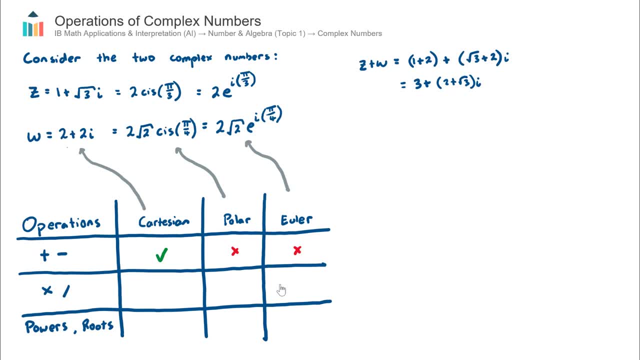 see. oh okay, it's probably a little bit easier to just multiply in either polar or Euler form. Let's start with multiplication in Cartesian form. So z multiplied by w will equal zero, The z complex number one plus root three, i multiplied by the w complex number two. 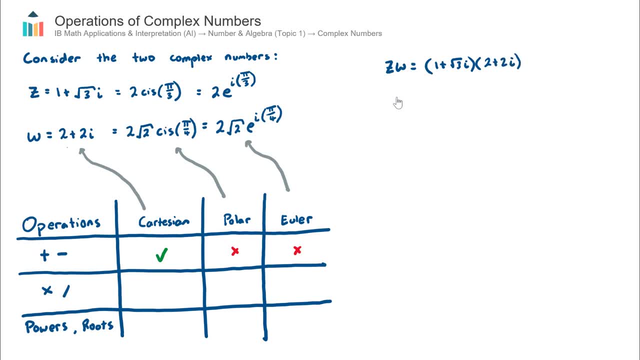 plus two i, And then we just expand these out or multiply these out by multiplication of two binomial turns. You would have done this plenty of times before. Recall the acronym FOIL: first, outer, inner, last. Let's go through that process. So I multiply one by two which. 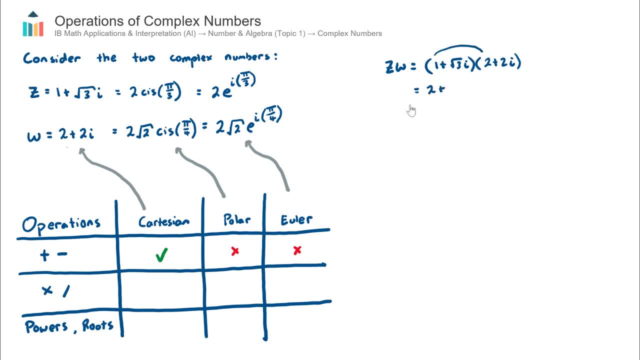 is just two Plus let's do the outers now. One multiplied by two, i, which is just two i. Let's do the inners: Root three. i multiplied by two will be two root three i. Finally, the last. just be careful with this one, it'll. 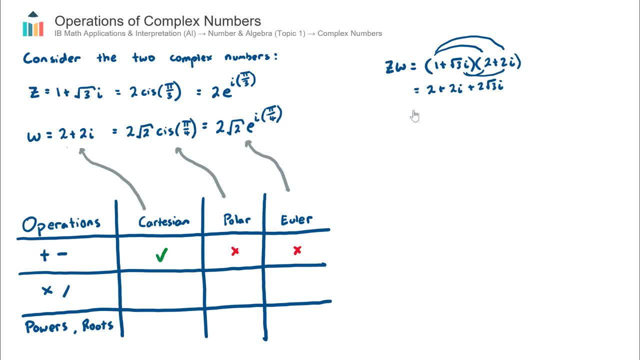 be root three. i multiplied by two i. So that will be plus two root three: i squared. Now just recall that i squared is equal to negative one. So therefore, if I group like turns and this, this will be two. Let's have our real components at the start, So it'll be two. 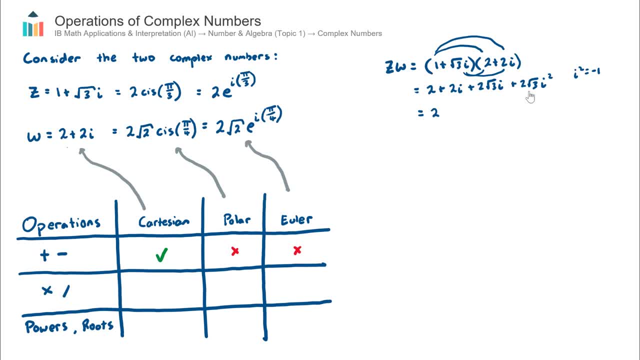 And this final component here will actually be subtract two root three, because the i squared turns into negative one. So this will be two subtract two root three And for the imaginary components I'm going to factor out i, So this will become plus I can actually. 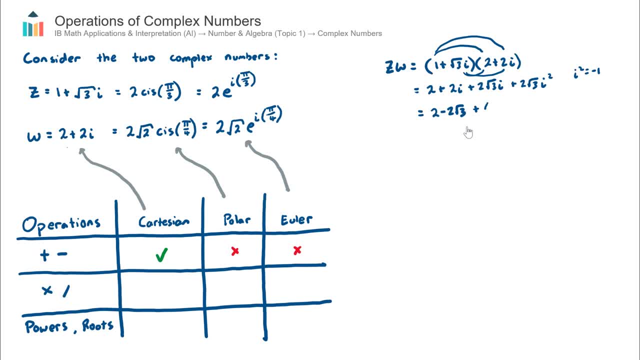 also factor out. ah, I won't factor out the two. This will become two plus two root three i. So you can see there that that wasn't too difficult. It only took a couple of lines of working. But if I had another complex number it would start to become quite long and tricky. 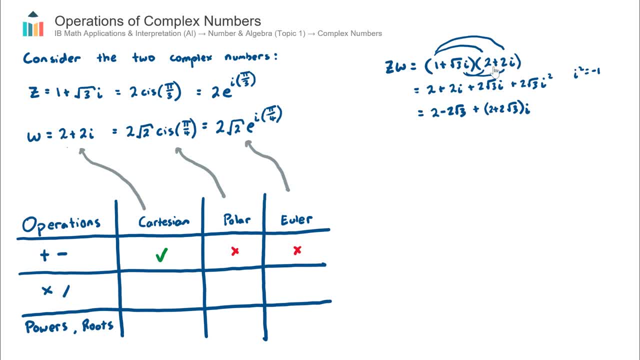 and also error prone. So just be careful with that. Let's compare that against multiplying two complex numbers in polar form. So z multiplied by w, that will equal. it'll be the modulus of z multiplied by the modulus of w, cis, and then I just add the angles together. So 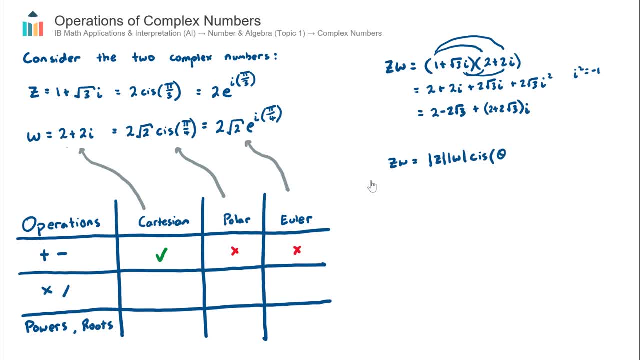 the arguments together, So the argument of z plus the argument of w. So you can see here: wow, that's quite easy. And even if I had three complex numbers, it would just be the modulus times, the modulus times, the modulus cis, angle plus angle plus angle. Pretty neat. 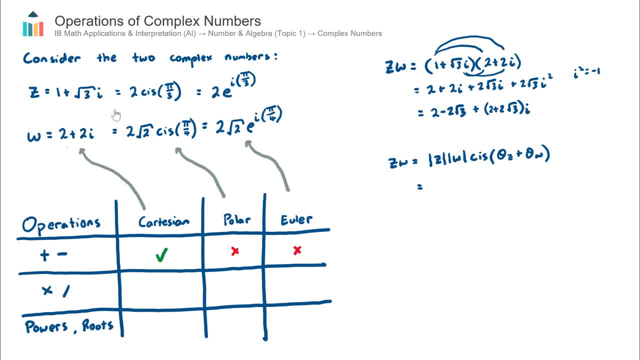 So this is, the modulus of z is two and the modulus of w is two root two. So that'll be four root two cis, and the arguments are pi plus two, Pi on three and pi on four If I add those together, taking a common denominator of 12,. 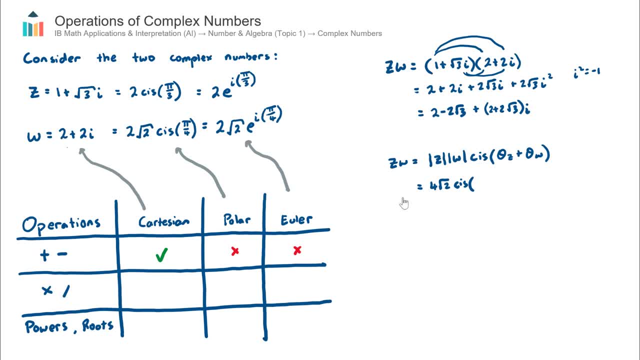 I will get seven pi on 12.. So there we have it. There is the multiplication. Now the answer will be in polar form, but you can see here that that's quite simple. Let's now do it in Euler form. So z multiplied by w will equal the. again, the modulus of 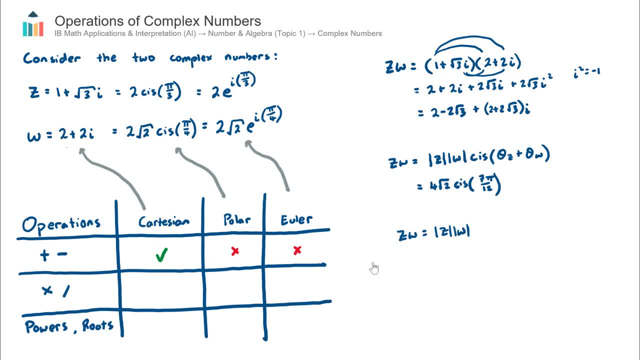 z multiplied by the modulus of w, e to the power of i, and then the argument of z plus the argument of w, So very similar to polar form, just in Euler format. So this will be four root two, e to the power of i, seven pi on 12.. 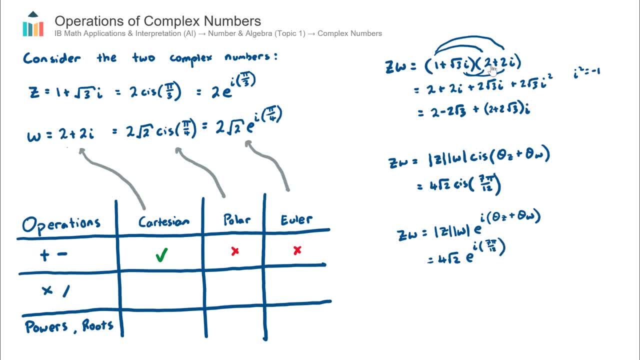 Okay, so that was multiplication. Let's now talk about division. Let's divide the complex number z by w in Cartesian form, and you'll see that this will become a little bit sort of complicated. It can be done particularly just with two complex numbers, but it does. 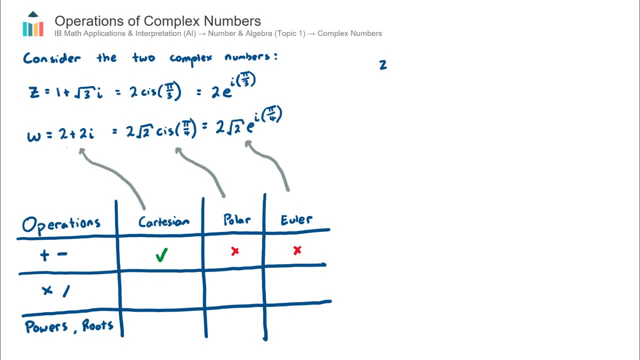 become a little bit tricky. So if I were z divided by w, that will be equal to, so one plus root three, i divided by two plus two i. And the way that I perform this division is: I multiply this fraction by another fraction, which is the complex conjugate of the bottom. 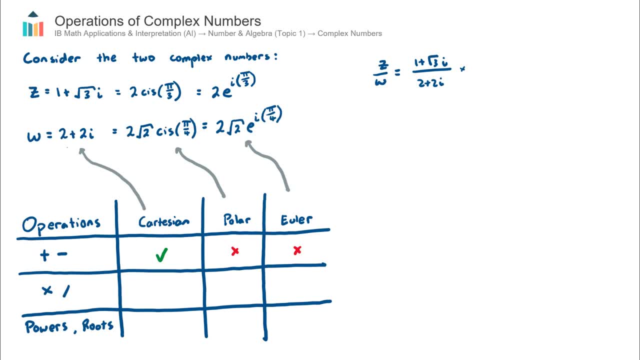 complex number here. Now I won't go into the detail on what that means, but it's essentially the same thing, but with the opposite sign in the middle. So if it was addition, it's now subtraction. That's called the complex conjugate. So I multiply it by this fraction. 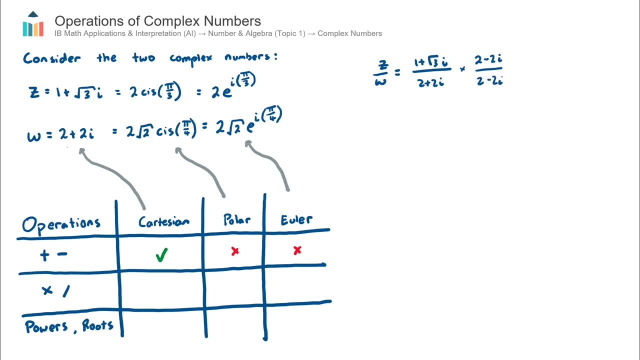 here, And the benefit of that is, if I multiply now the numerators together, by multiplying two binomial terms and the denominators together, we'll end up with a real denominator. It won't be a complex number. Now I won't go ahead and do this because that will probably take. 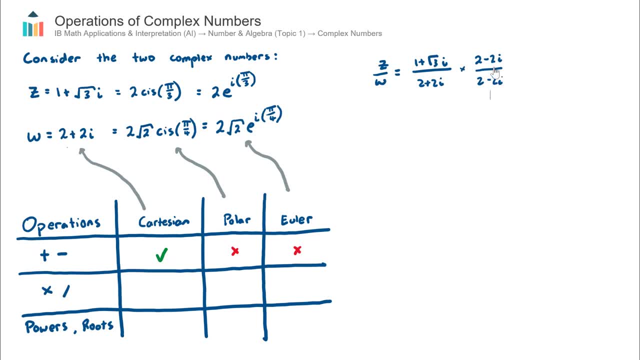 me five to ten minutes. I don't want to waste your time doing all that algebraic expansion, but you can see here that that will become quite tricky. Let's now compare that with the division of Z by W in polar form. So Z over W. 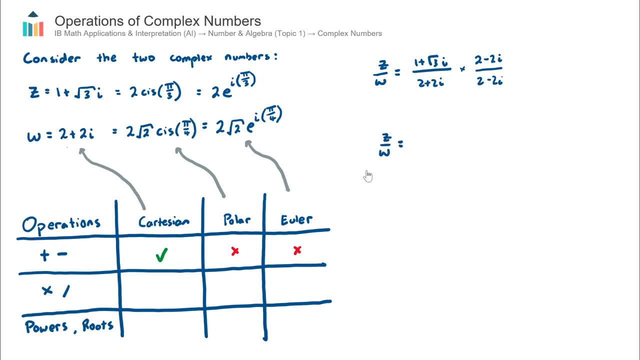 Is equal to. it's kind of the opposite to the multiplication. It'll be the modulus of Z Divided by the modulus of W, Sis, and instead of adding the angles, like we did for multiplication, We're actually going to subtract the angles. The arguments are- I keep saying angles, the proper, correct word is argument. So the argument of Z. 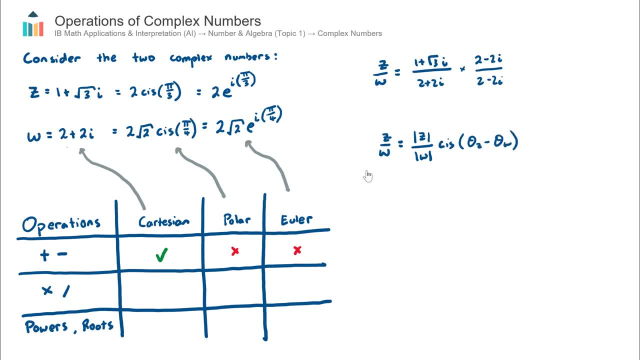 subtract the argument of W, So that will equal net. so the modulus of Z over the modulus of W, So it'll be 2 divided by 2 root 2.. I can just simplify that in my head to just 1 on root 2, Sis and. 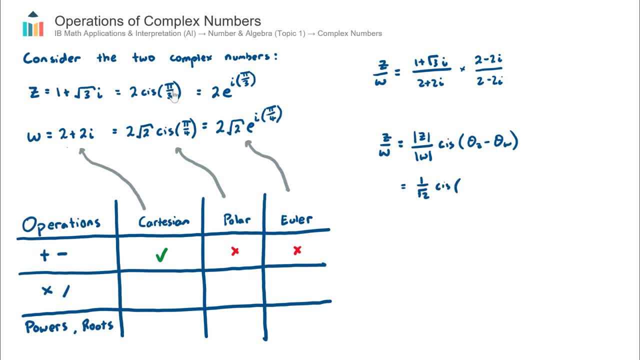 The argument of Z is PI on 3 subtract PI on 4.. Let's make a common denominator of 12. It'll be 4 PI On 12 to subtract 3 PI on 12. It'll be PI on 12. So quite simple there. and that works exactly the same for Euler form as well. so Z over W will equal. 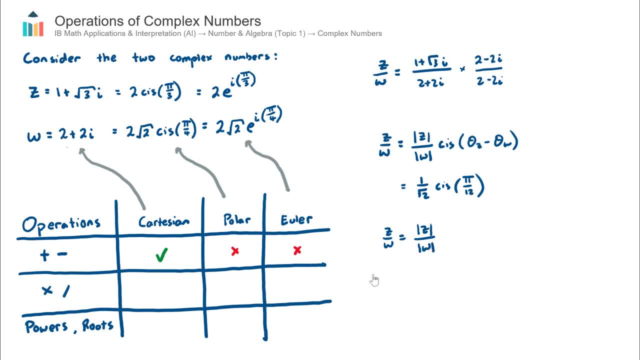 The modulus of Z divided by the modulus of W e to the power of I, the argument of Z Subtract the argument to W and that will equal 1 on root, 2 e to the power of I, PI on 12. so very similar for polar form and Euler form. 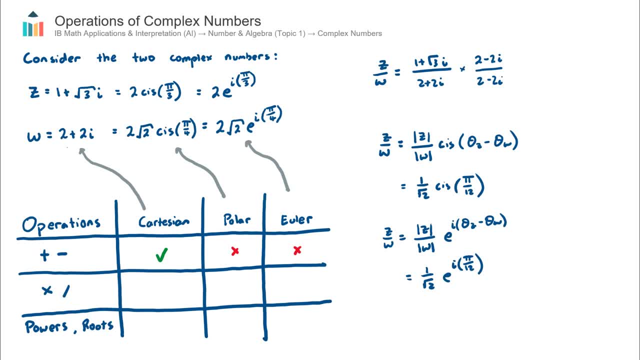 So to summarize my findings on the table here, I'm going to put a sort of Swiggly orange line here for addition, for multiplication, division, for Cartesian form. so proceed with caution. But I'll put two ticks here for polar form and Euler form. Okay, let's now finish off by looking at the taking, the power of a complex number for these three forms. 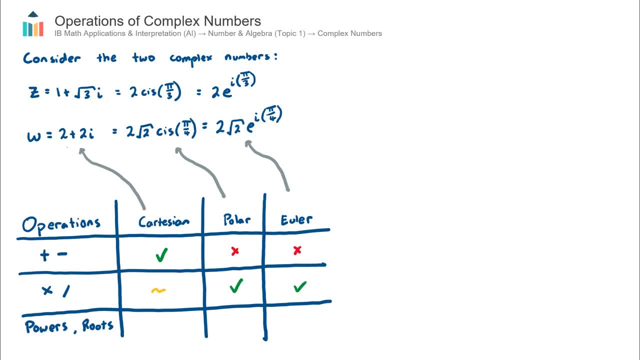 Let's say that I wanted to raise the complex numbers Z To the power of 4. So this complex number here I want to raise it at the power of 4. Well, in Cartesian form what this would look like: I would have to go 1 plus root 3i. 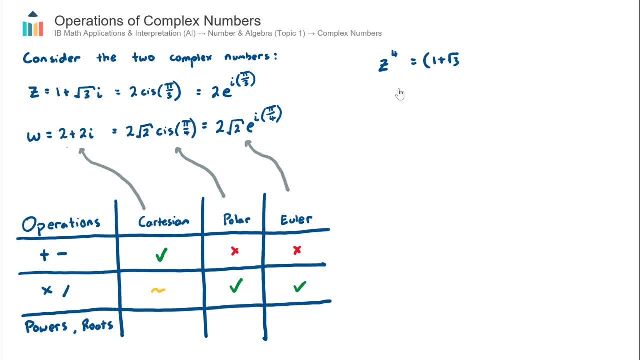 Sorry, root 3i Multiplied by 1 plus root 3i Multiplied by 1 plus root 3i Multiplied by 1 plus root 3i. So I've done that four times to the power of 4, and then I need to expand this all out and you can see here: 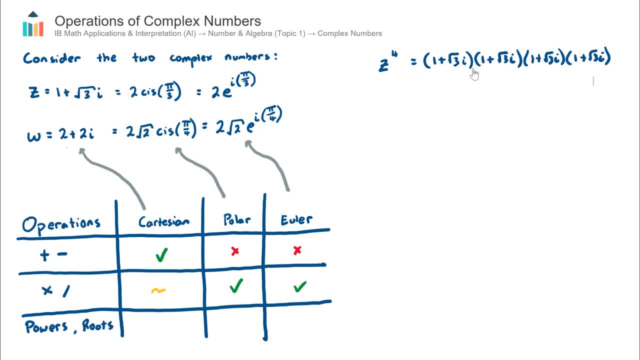 Wow, that would take a long time and very prone to making a mistake. I need to be expanding binomial turns four times, So not a great method to take powers or complex numbers. I'm going to put a cross here against powers in Cartesian form. Let's now compare that to polar form and Euler form. 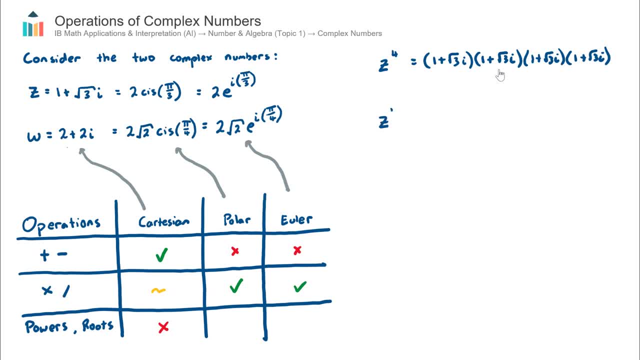 So if I went Z raised to the power of 4 in polar form, What I can do is I can take the modulus and raise that to the power of 4 and then put cis, Take my angle and multiply it by 4.. Sorry, not raised to the power of 4, just multiply it by 4. 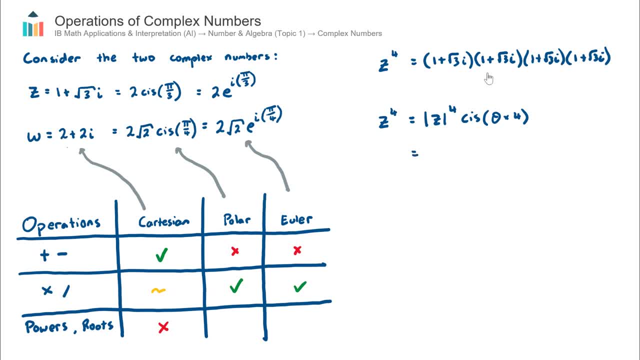 So this would become the modulus of Z is 2.. So 2 raised to the power of 4 is 16. so it'll be 16 cis, and My argument is: pi on 3, multiplying that by 4. I'll get 4, pi on 3. 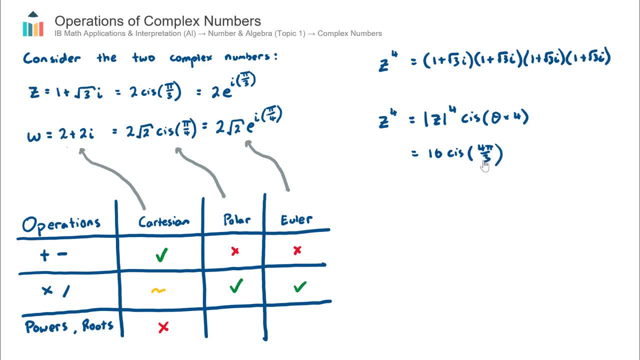 So look at that, quite simple to raise powers in polar form, And likewise for Euler form. let's have a look at this one here. So Z to the power of 4 will equal the modulus of Z raised to the power of 4, e to the power of i, and again the argument multiplied by 4. 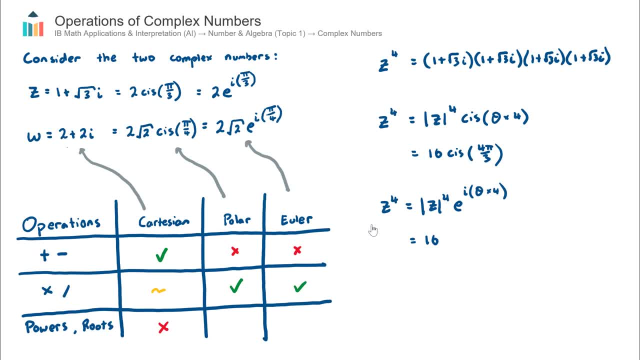 That will equal 16 e to the power of i. and again The argument is: pi on 3 multiplied by 4 gets 4 pi on 3. So you can see there that polar form and Euler form is very, very useful for finding the powers and 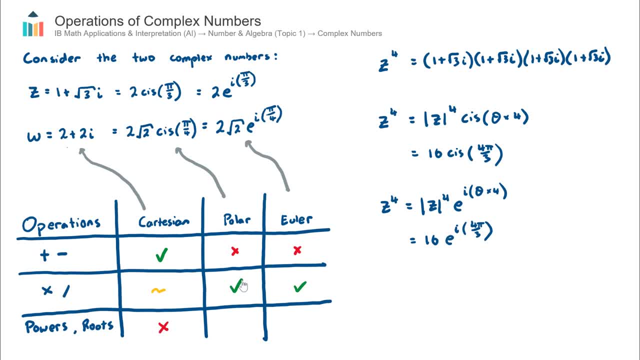 Likewise for roots. roots works exactly the same, just except the power will be, say, 1 on 3 or 1 on 5 for, say, the cubed root or fifth root, It'll work exactly the same. So I'm going to put two green ticks next to polar form and Euler form for finding powers and roots of complex numbers. 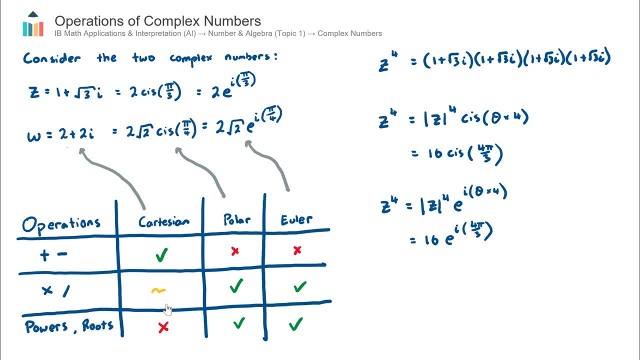 Okay, that concludes our overview video. video there: I highly recommend practicing these operations in the different forms. Yes, but that concludes our video on operations of complex numbers.